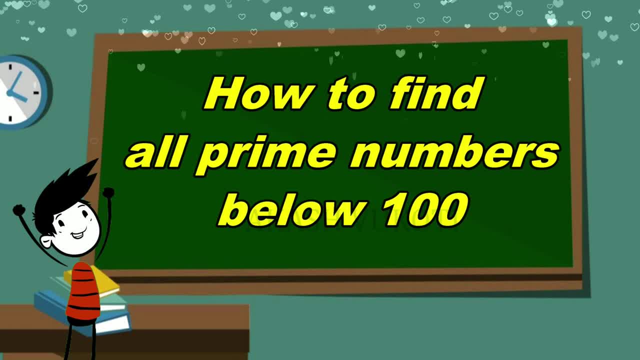 trick that are going to be helping you whenever you need prime numbers. And as prime numbers are a very important concept in mathematics, learning how to identify these is perhaps one of the most important things. So let's take a look at how to identify all of the prime numbers under 100.. A prime number is a. 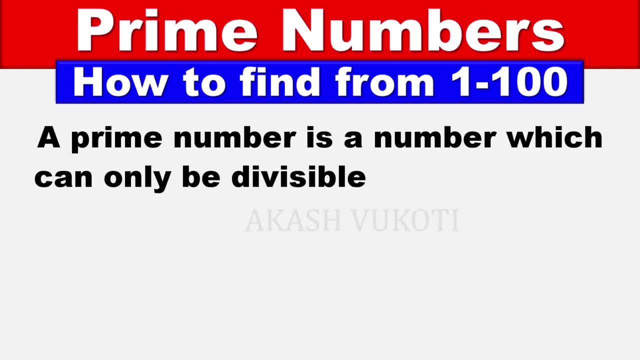 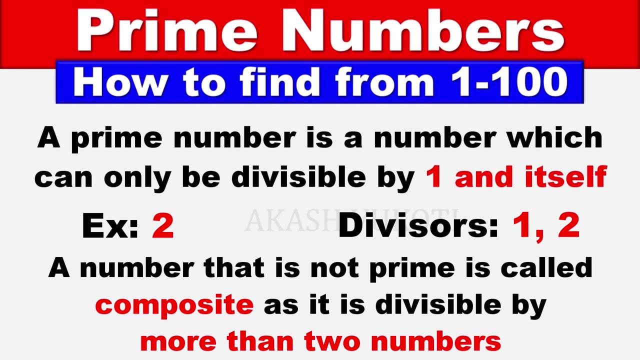 number which can only be divisible by 1 and itself. As an example, the number 2 is prime because it can only be divisible by 1 and itself, which is 2.. A number that is not prime is a prime. It is called composite as it is divisible by more than two numbers. Now let's deal. 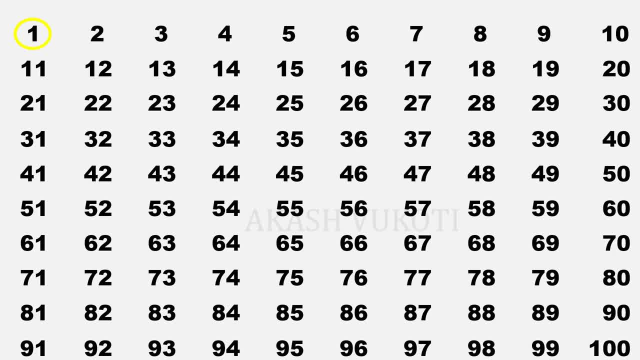 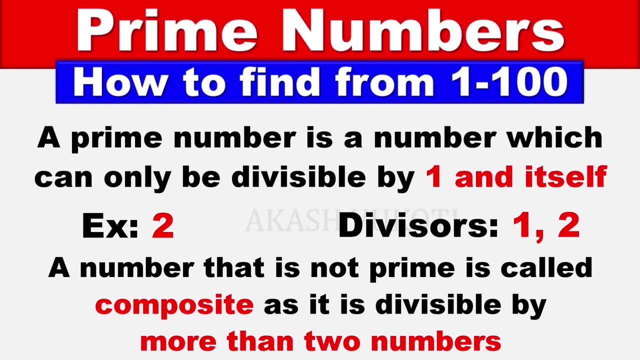 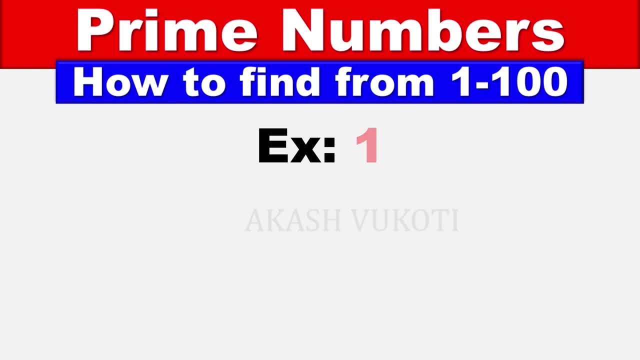 with the special case of the number 1, because a prime number has to be divisible by two numbers and a composite number has to be divisible by more than two numbers. So if we take a look at the number 1, it can only be divisible by 1. 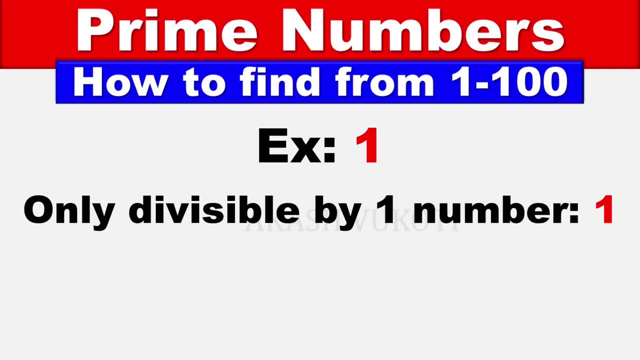 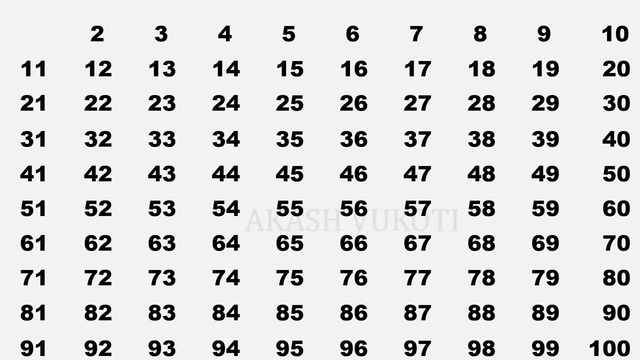 number, which is well, 1.. So is it prime or is it composite? Well, as it turns out, 1 is neither prime nor composite. It is in its own special category. So now, now we're ready to take a look at the sieve of Eratosthenes, otherwise known as how to 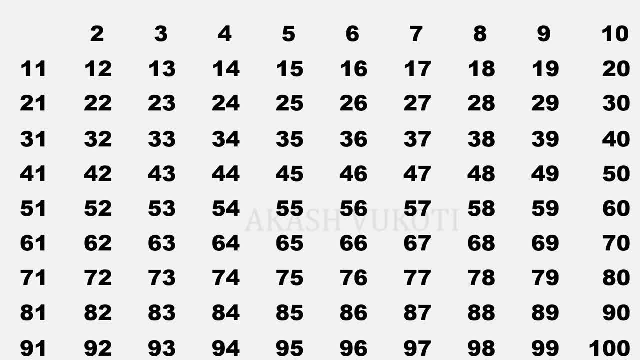 find all the prime numbers below 100.. Let us begin By arranging all of the numbers, from 2 all the way up to 100.. We're ignoring 1 here because, as we have mentioned, 1 is neither prime nor composite. It is in its 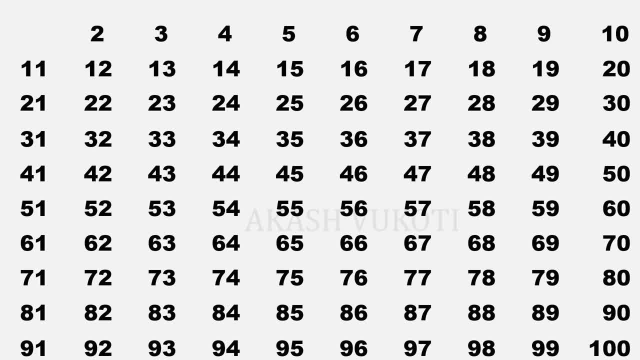 own category. So let's take a look at all the numbers from 2 to 100.. We begin by circling the number 2.. It is going to be our very first prime number. Now, after this, we have to cross out every subsequent multiple of 2 from this list. 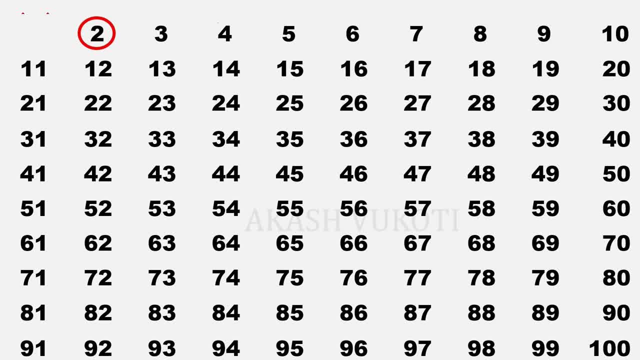 because they are not prime, as they would all be divisible by 2,, therefore composite. So let us cross them all out now. As you can see, we can now start crossing out 4,, 6,, 8,, 10, and all of the other numbers divisible by 2, which. 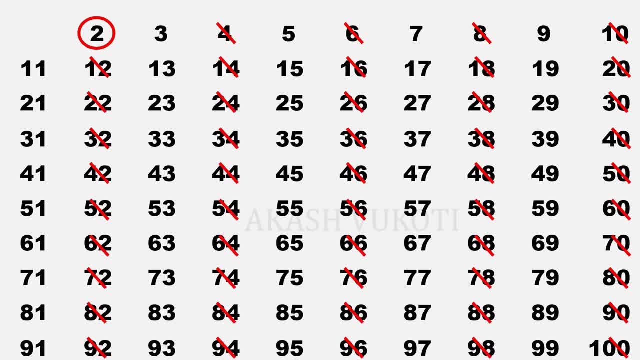 are not prime because, as well as 1 and themselves, they're also divisible by 2 as well. So now that we have successfully crossed out all of those multiples of 2, as you can see right here- we can now see that our next prime number is the one. 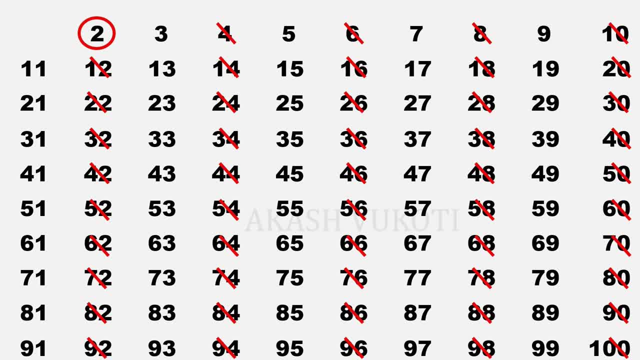 that has not been crossed out yet, which is 3.. So we will circle 3 as our second prime number, and then we will cross out every subsequent multiple of 3.. Now you will see that some of these are also divisible by 2, and for those we can just leave them as they are, which is crossed. 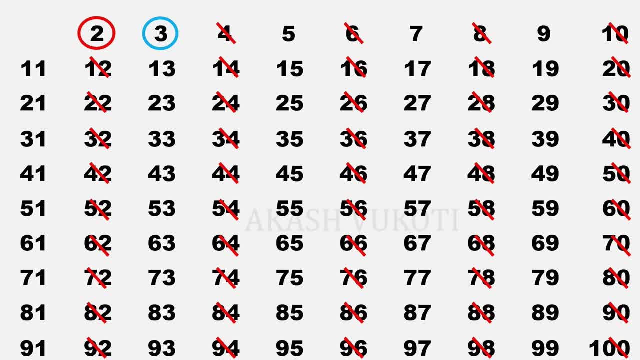 out and just cross out all the unique ones that haven't been crossed out yet. So, as you can see, we have crossed out 6,, 9,, 12,, 15,, 18, and so on, through all of the multiples of 3, which are not prime and are instead composite, because, aside 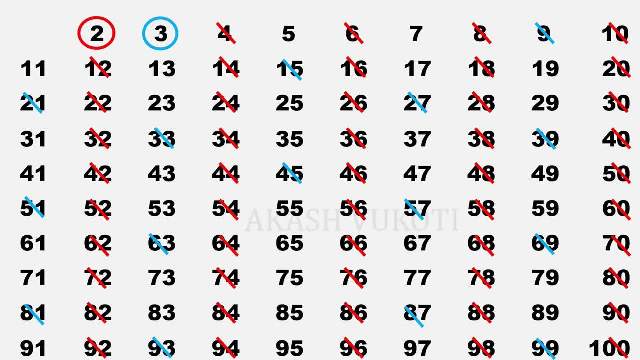 from 1, and themselves they're also divisible by 3.. Next up, you can see that the next number we have not crossed out yet is 5, and so we will circle it as our third prime number, and then we can simply cross out every multiple of 5. 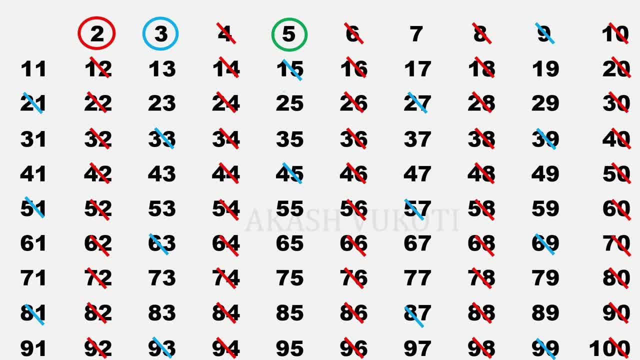 afterwards. So this includes 10,, 15,, 20,, 25,, 30, and so on, And, as you can see, a lot of those have already been crossed out from when we did 2, but that's no worry. 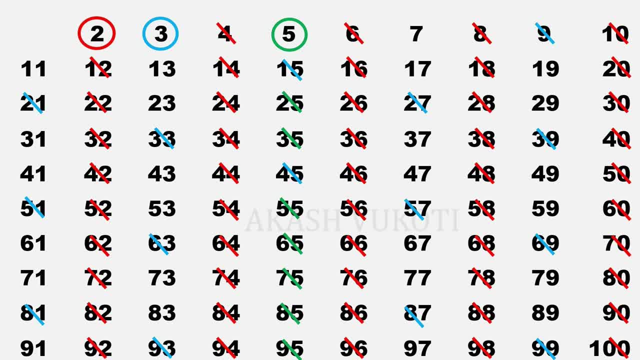 because, as they have already been crossed out, we can just cross out the ones that are unique. and now we are almost there, And now all we have to do is take a look at the next number that we have not crossed out yet, which, in this case, is 7.. So 7 is our fourth prime.